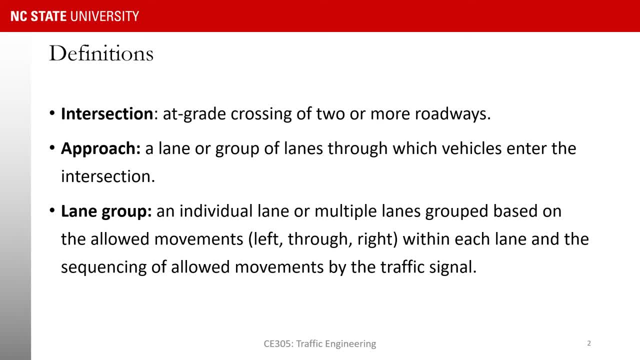 And this word at grade is the key word here. So if you have one roadway that crosses the other one not at the same level like an interchange that you see on a freeway, that's not going to be the focus of this chapter. So intersections are at grade: crossing of two or multiple roadways. 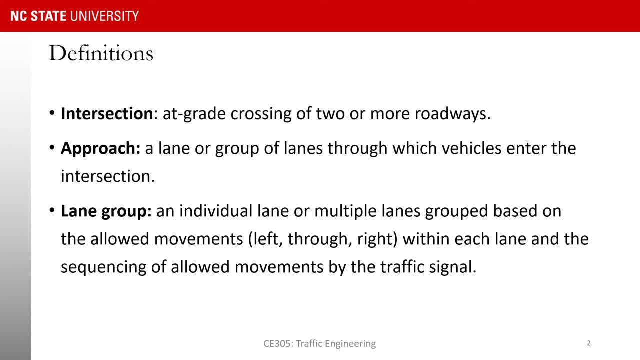 The other definition is the definition of approach. Approach is a single or group of multiple lanes that are used by vehicles to enter the intersection. So think about an intersection of two roadways and each of those roadways. In such an example you have two approaches because vehicles use two different places to enter the intersection. 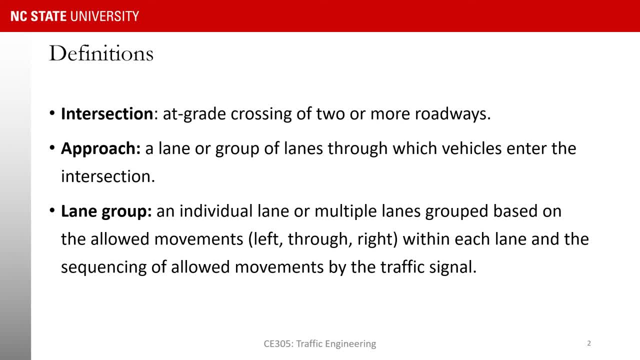 If you have an intersection of two two-way streets, then you would have four approaches, as vehicles are using four different places to enter the intersection. The other definition that we use over and over again is the definition of intersection. that I would like to cover on this slide is the definition of lane groups. 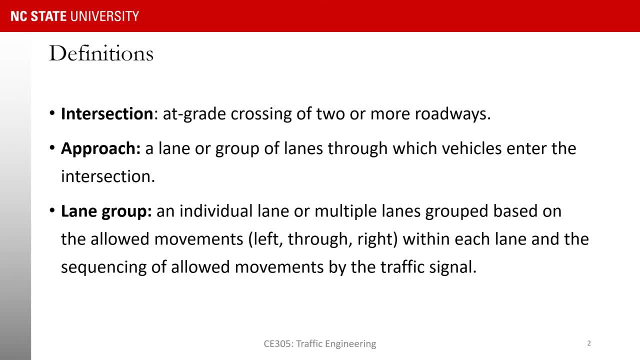 So a lane group is either a single or multiple lanes that are allowed to go through the intersection at the same time, and usually these lanes are served by the same phase and they have the same saturation flow rate to process vehicles. We talk about lane groups further later in this chapter. 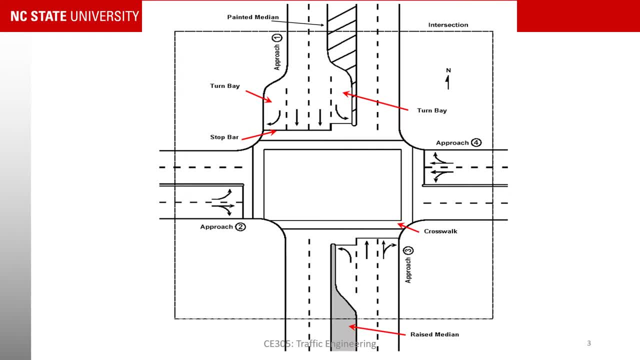 What I have on this slide is a layout of an intersection, So you can see that this is an intersection or crossing of two roadways. Each of those, each of those roadways are two-way. So what we have here is four approaches, as you can see on the. 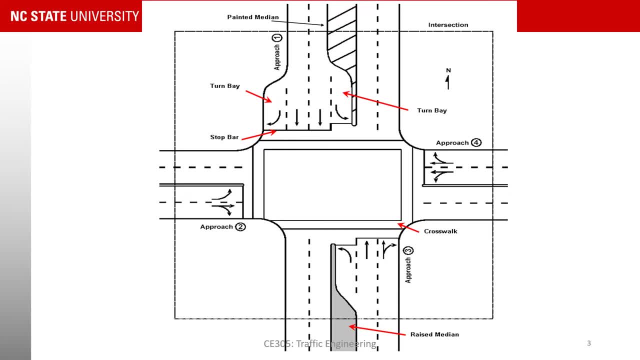 figure by approach one, two, three and four, And for a few minutes I would like to focus on approach three. Here you can see that I have two lanes and a left lane path. So if I want to talk about lane groups here, I have three lane groups. 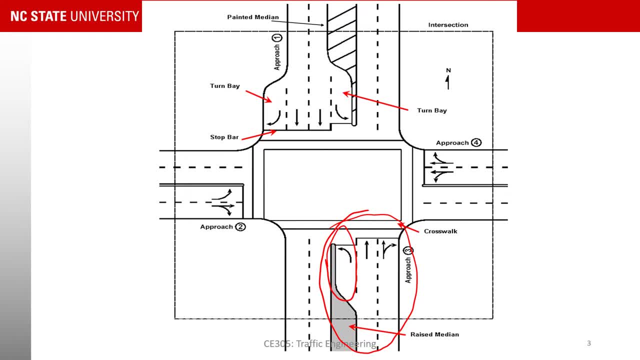 One lane group is this group of vehicles that are making a left turn. The other group is this group of lanes that are going through And the last one is this group on the right that are either going through or making a right turn. Now you need to. 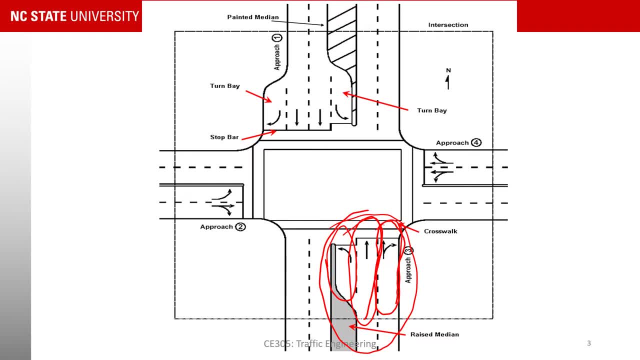 keep in mind that this lane is a shared true and right lane, So let's focus on approach one. Here also, I have three lane groups, While if you take a look at the number of lanes and pockets together, those are four. So one lane group here is making a right turn. The other lane group 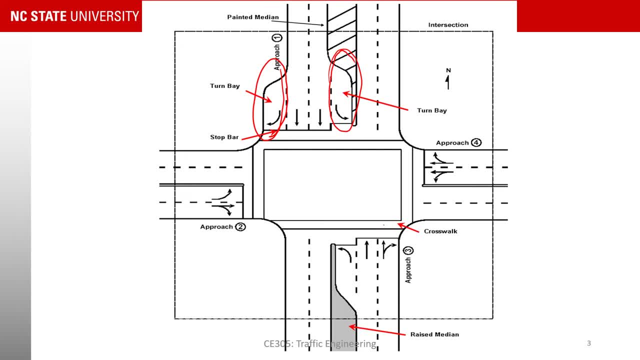 is for vehicles that are making a left turn, And then these two lanes are grouped together And this is a lane group for those lanes that are used for vehicles to go through the intersection. So here I still have three lane groups. On this figure also, you can see the stop bar, you can see turn bays. 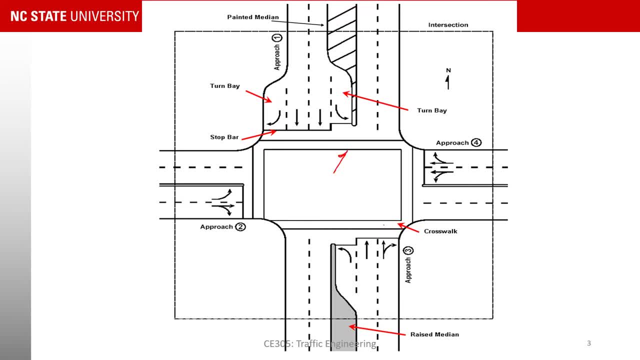 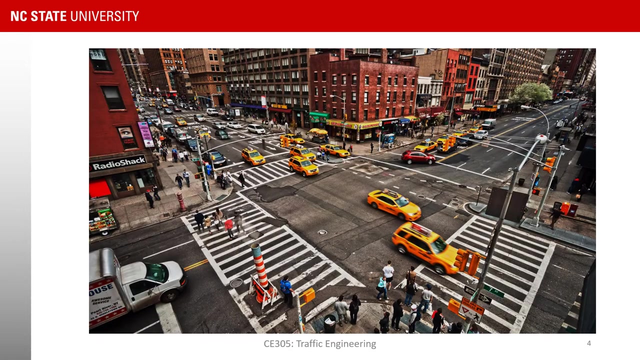 you can see pedestrian crossing, you can see medians and other things at an intersection. I would like for you to take a look at this figure and think and think about things that are going on at an intersection. So let's take a look at this figure and think and think about things that are going on at an intersection. 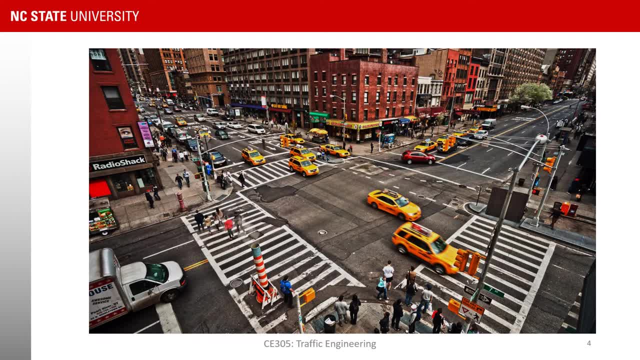 Some of the things that make the analysis of this intersection challenging. so, for a few seconds, think about things that create complications in analyzing what is going on in this intersection. For instance, if you think about this intersection, you will see a lot of pedestrians that are present in the intersection neighborhood, so the interactions that they have with vehicular 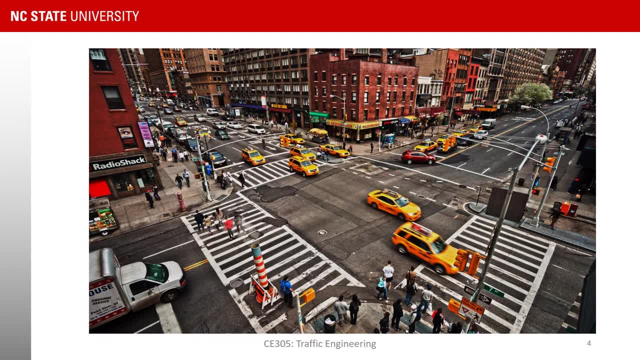 movement is going to create complications. another thing that you can see here is the number of taxis that are present. so why do you think taxis are going to create complications? because they're going to stop to pick up or drop off passengers, so that's going to create. 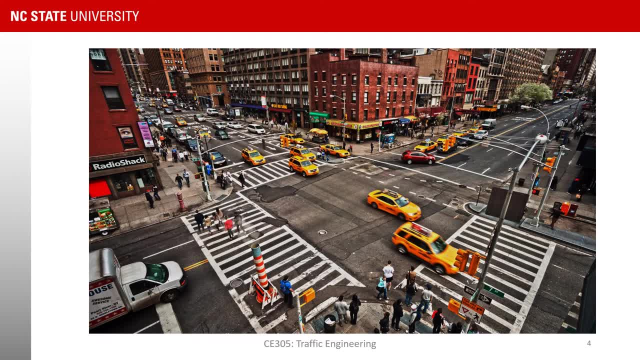 some disruption to traffic flow when you go to the intersection. how about other things? you can see that this lane is closed. here. there is some construction happening in this intersection, so that is going to create, that is going to close one of the lanes, so not only one lane is closed. 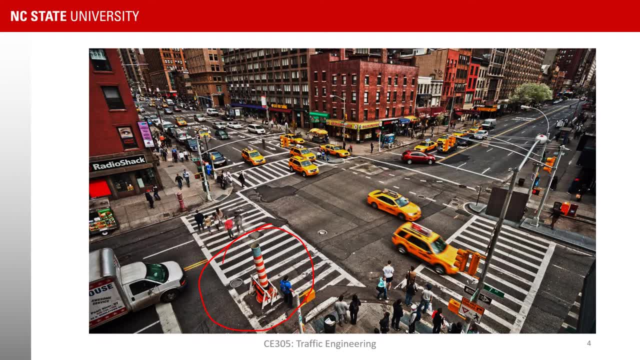 now vehicles upstream of that lane need to plan for future and they need to pretty much change their lane. so you really see a couple of complications there. one lane is closed and then you're going to have some unplanned lane changes in this intersection. if you also 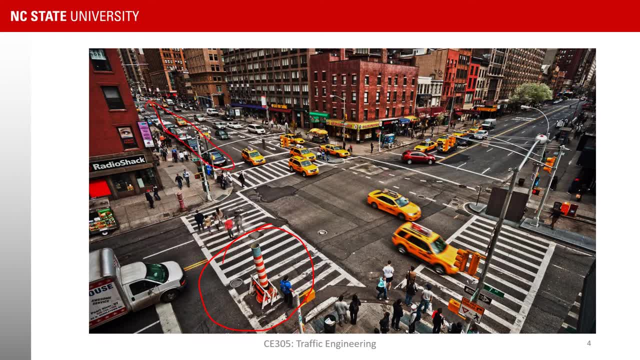 take a look at this side, you can see that a number of vehicles are parked, so does that create any complication? the answer is yes, these vehicles, when they want to park, they're going to block one of the lanes for some time. when they want to get out of the parking. 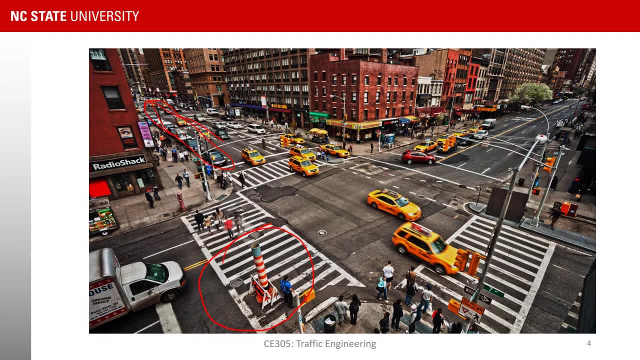 spot, they're going to do the same and that's going to create some problem and you're going to lose some of the capacity of the intersection, and there are other things like that that you can see here that makes the analysis of a signalized intersection a very complicated task. 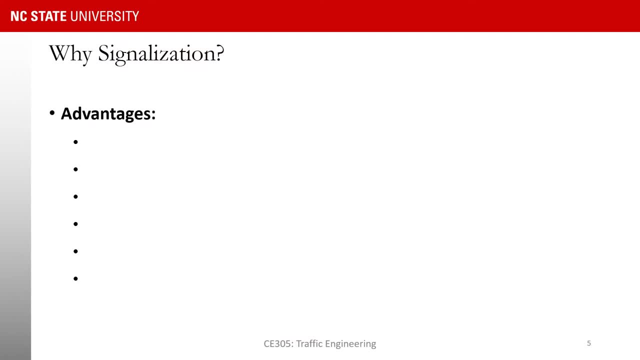 so here i would like for you to think about some of the advantages of signalization, or think about why we would like to install signals at an intersection rather than having stop signs or other forms of controlling the traffic. so what are some advantages that we hope to achieve from signalization, and i would like for you guys to 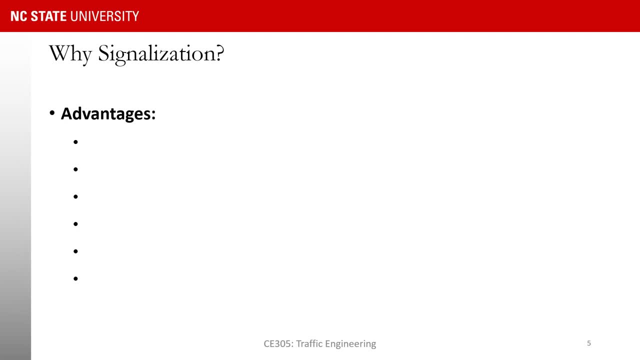 to pause the video here for a few seconds and think about it and then continue with the video. so if you think about, one of the most advantages of signalization is the reduction of some types of crashes. so why do we put signals at an intersection? because we 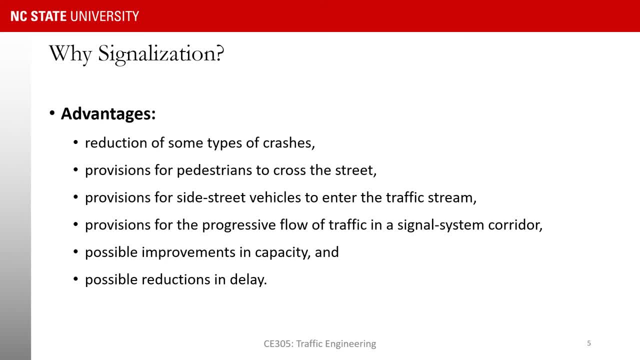 don't want two movements that have a conflict to go through the intersection at the same time. think about a vehicle that is going from north to south and a vehicle that goes from east to west. if they enter the intersection at the same time, there is a hard, there is a high chance for a crash. 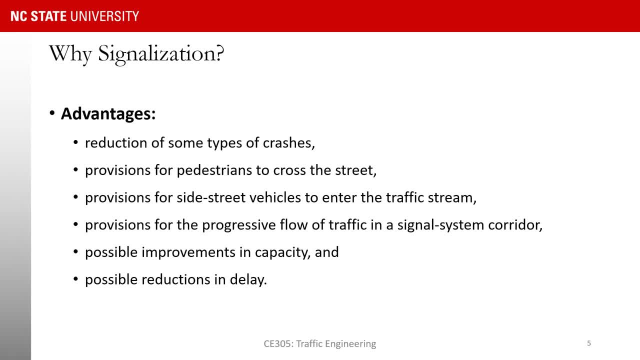 so if a signal is done properly is gonna reduce or eliminate the probability of these types of crashes. a good signal can help pedestrians to cross the streets at the intersection, so it's it will provide them with enough time to pass the streets safely. also, it can provide the possibility for traffic from side street to enter. 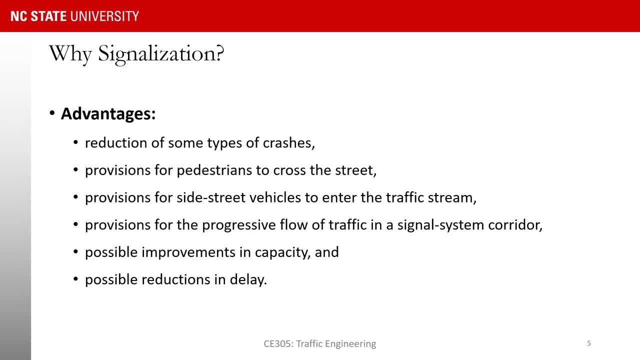 the traffic stream and go through the arterial or go through the intersection. think about an intersection of a major and a minor street where you control the traffic with stop signs on the minor streets. it's hard for traffic from minor streets to either cross or join the traffic on the major street if you just have stop signs, a properly timed traffic signal. 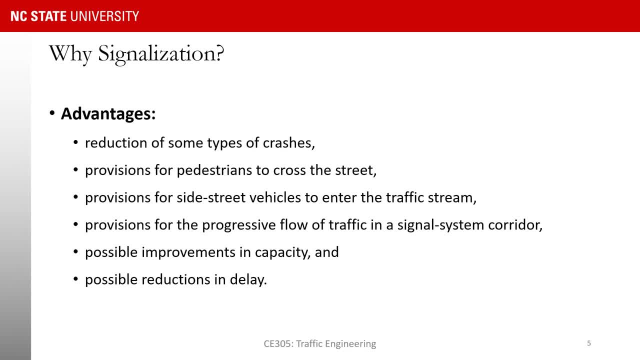 allows that traffic from side streets to enter or cross the intersection safely and efficiently. signals also, if they are done the right way, can provide possibility for coordinating for traffic if you have a distance from parte when there's an intersection. this is comfortable for some where, if you reserve, the room in the center of your would remain. 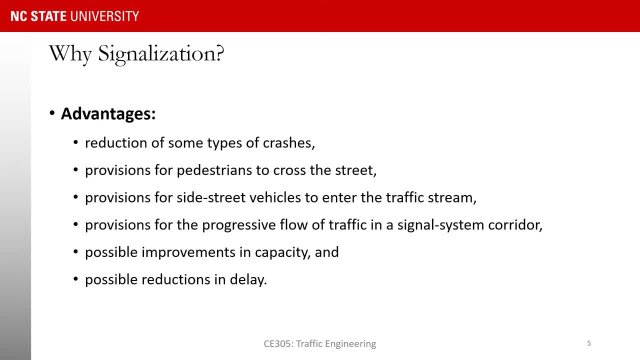 the way to litter the area. and someone else can: Sabine, які are Vägena? where you can, dennis, run them to the left of the club? wi-fi, maybeですね. it's a permanent one if you have it without my friend isrenky. 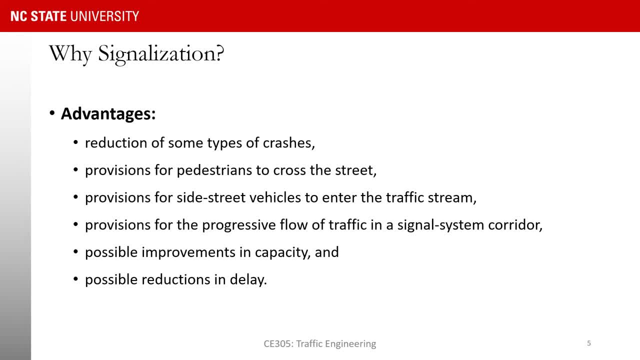 the signals are very well coordinated and after your signal turns green, you have a good chance of going through several intersections without stopping, and the vice versa is true when you're going out or when you're going to north through downtown in in the evening peak. so if signals are done properly, they can improve capacity and also they can 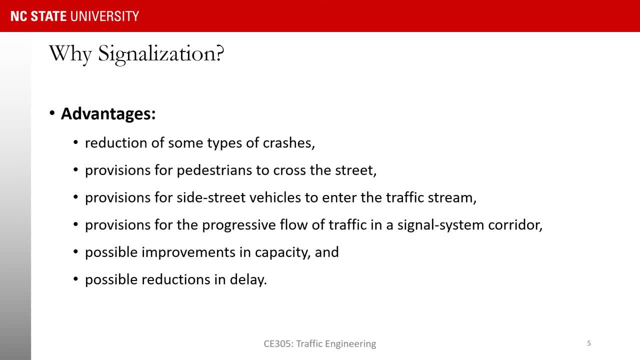 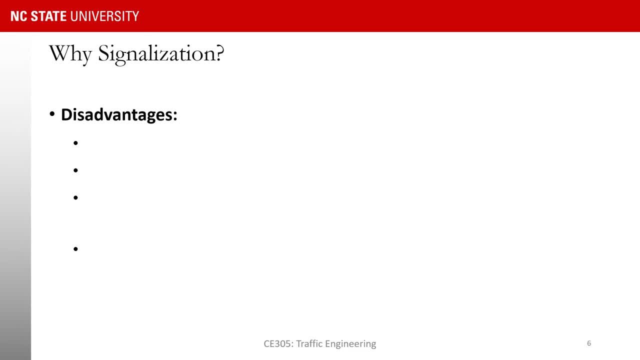 reduce the delay. but what if signals are not done properly? so what are the disadvantages of signalization if they are not done properly? so pretty much whatever you saw on the previous slide, you can think about those. you can think about those as a disadvantage. so you can increase vehicle delay. you may increase some. 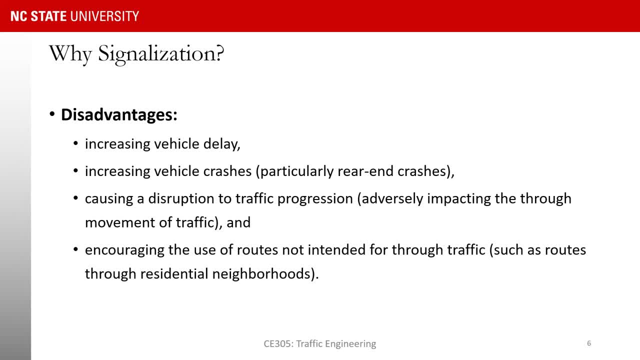 other types of crashes. for example, rather than- rather than having t-bone crashes, now you can have rear end crashes. if the signals are not done properly. rather than having a green wave or signal coordination, you may cause vehicles to stop at each the intersection when they're going through an arterial, and if that is, 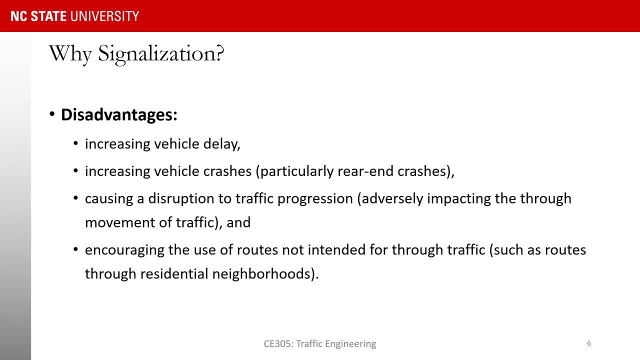 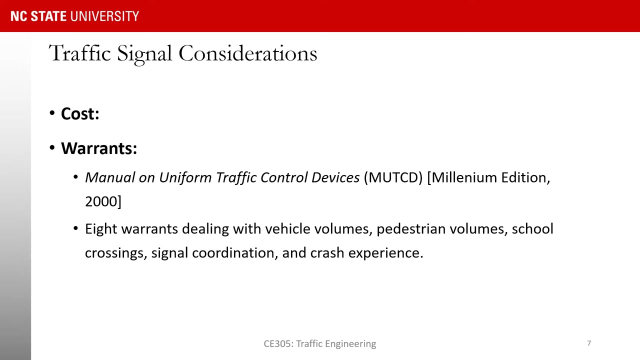 happening. you're pretty much encouraging traffic not to use that arterial and take some other routes that are not intended for that level of traffic, so that's also a disadvantage. so let's assume that in a perfect world we can design signals perfectly and we are going to have all the advantages and none of the. 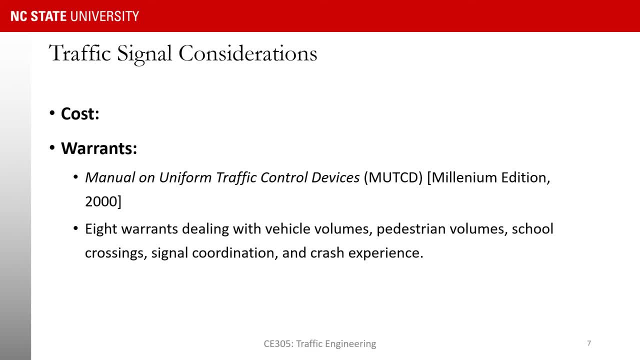 disadvantages in such a world. are we gonna put signals at each intersection? the answer is no and if you want to know what is the reason, the reason is the cost. so signalization is expensive if you think about typical cost to just install all the hardware and software that is required for. 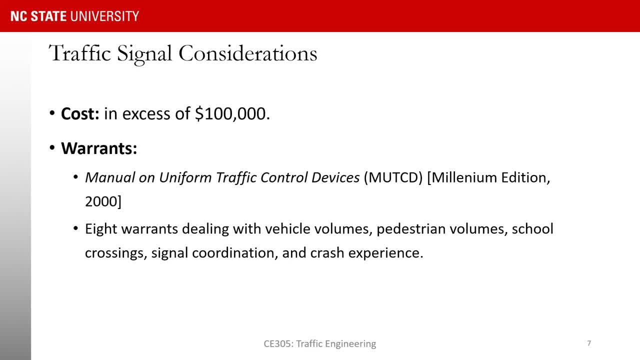 signalization at a typical intersection that is in the excess of one hundred thousand dollars. and we have many intersections, most of which are not signalized. so for that reason there are a number of warrants that need to be met so that we as traffic engineers go and install signals at the intersection and 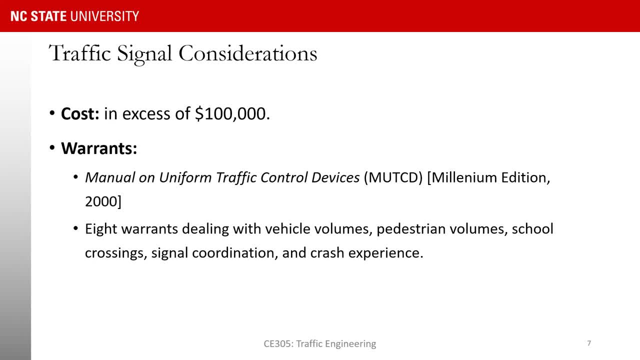 those variants are listed in the manual on uniform traffic control devices or mutcd, and there are a number of those variants that deal with volume, pedestrian volume, school crossing, signal coordination and crash experience. that is going to just be used to to justify together the need for installing a signal. we are not going to go through those. 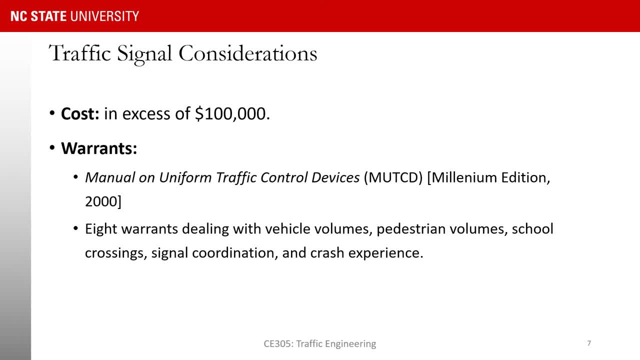 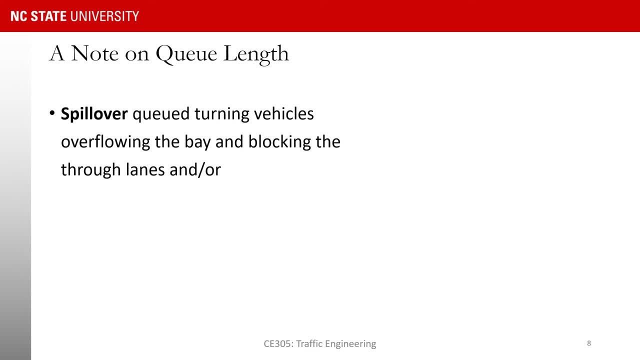 in this course, but in a follow-up course we will visit them. so i also want to have a note on the queue links. there are two concepts that i want to talk about. one is spillover and the other one is, and the other one is spill back, and one of the things 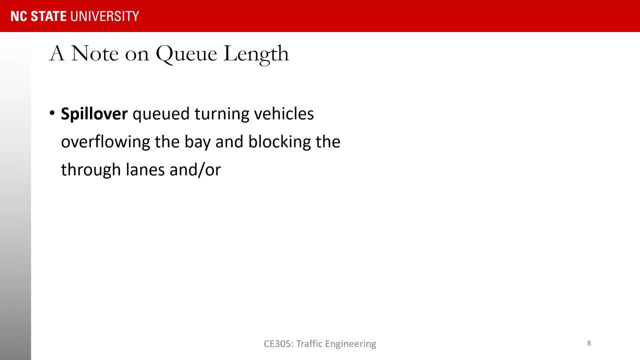 that we want to do with signals, and with properly design and time signals, is that we wanna eliminate spillovers or spillbacks. so here in this figure i'm showing you spill over: you're seeing that the queue and the left lane pocket has increased and spilled back to the true lane. so what it is doing, 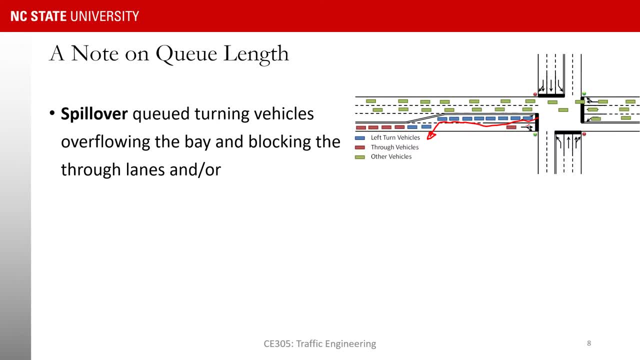 now is that it blocks the true lane and those two blue cars that want to make a left turn are gonna stop there and pretty much block the entire traffic to go through the true lane while you have, you know, capacity or enough space left on the true lane. so you're gonna have starvation when the signal 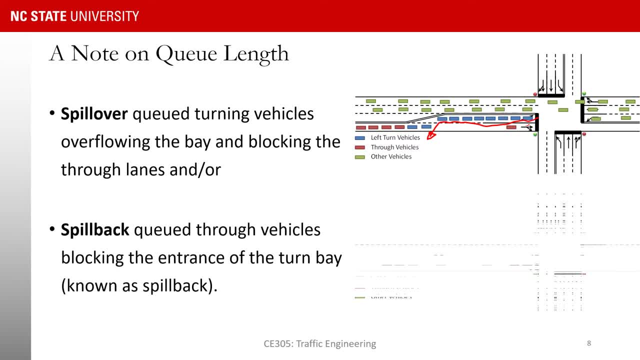 is green, we want to eliminate that. spill back also needs to be eliminated. so now you will see that the true traffic queue is long and it is pretty much past the pocket, the left turn pocket. so that blue car that is left here doesn't have a chance to join this lane and go through the intersection. 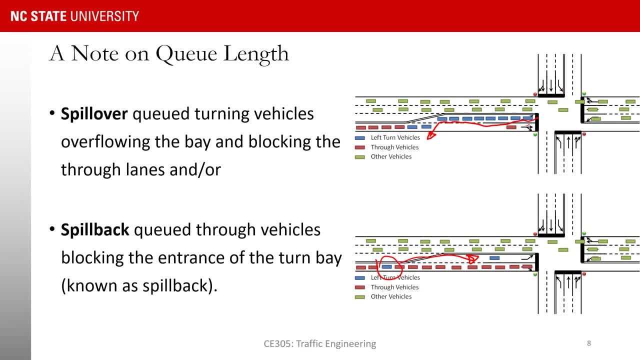 if there is enough gap or if there is a left turn arrow for that movement. so the queue from true movement is spilled back and has pretty much eliminated the possibility of that car to join the left turn pocket. we want to eliminate that. so a properly designed signal. 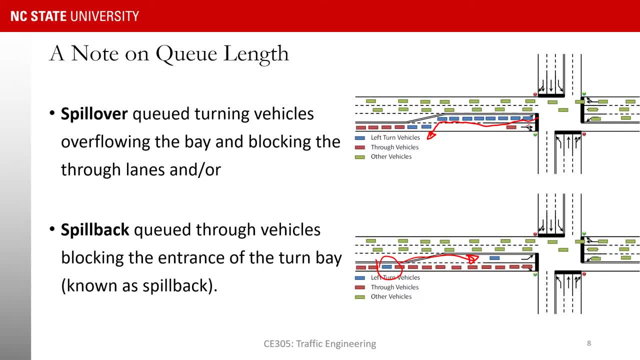 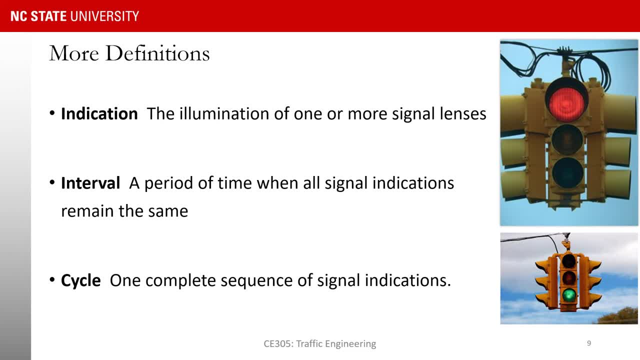 should eliminate both spill back and spill over. i have more definitions that i would like to share with you. we have indication, so here in this figure, you're seeing a red indication. so what are we going to have at a signalized intersection? we can have a green indication, we can have yellow indication and 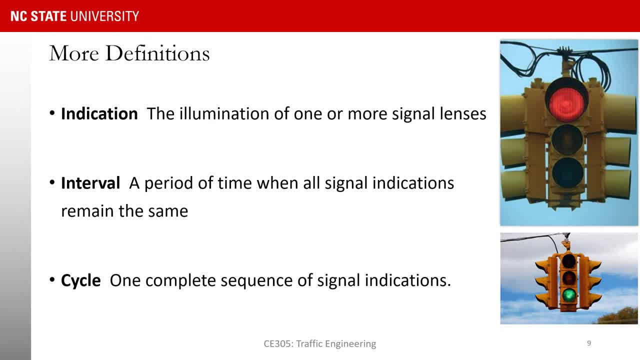 red indication interval is a period of time when all the signal indications are the same or you don't see any change in any signal indication at. the intersection cycle is one complete sequence of signal indications. for example, in the signal head that we are seeing here, if the green starts at t equal to zero and then stays green for, let's say, 50 seconds, then 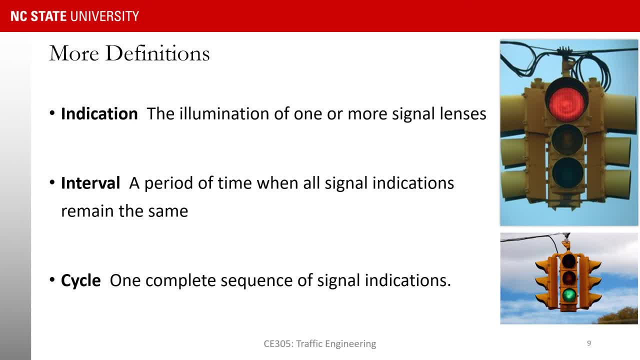 it turns yellow for 5 seconds and then turns to red for 20 seconds. after 75 seconds, which is the summation of 50 plus 5 plus 20, we are going to see the green illuminated on this signal head again. that is defined a cycle and that 75 seconds is defined as cycle lengths. 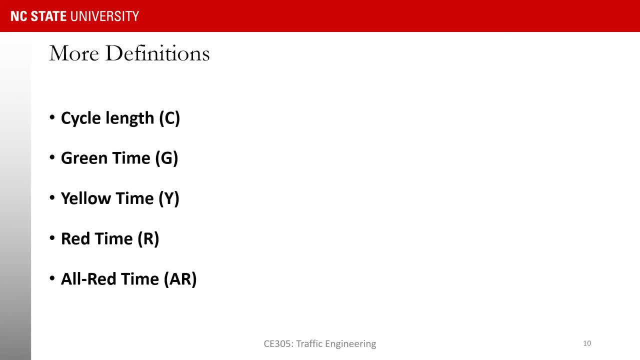 so we show cycle lengths with capital c: green time with capital g, yellow time with capital y, red time with capital r and all red time with capital a and capital r. can you think about the need for for all red time? why do we use all red? well, we use all red to allow vehicles that enter the intersection before the signal. 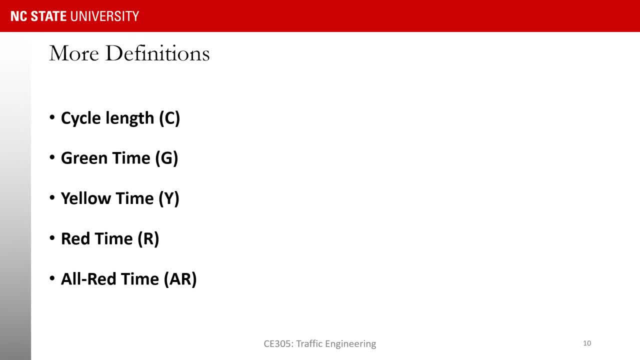 turn red to clear the intersection. so we show red signals to all different movements so that no one comes in and those that are inside the intersection can leave. can you think of a typical duration for all red? it's usually between one and two intersections and the duration also depends. 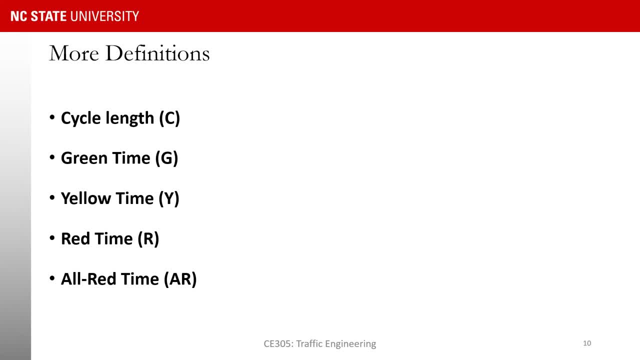 on the widths of intersections or streets. so on this slide i would like to talk about different types of controllers or control logics that we use at signalized intersections. you see three different controllers: pre-timed, semi-actuated or fully actuated control. so pre-time are those controllers that the timing is given to them and the timing can change from. 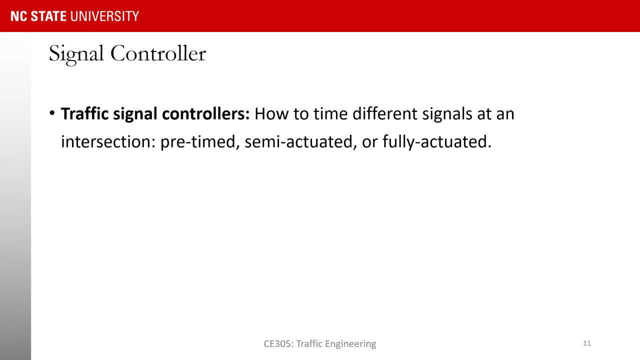 let's say morning peak to evening peak, but during each period it is fixed. if you have more vehicles arriving during that period, signal timing does not change. if you have fewer vehicles arriving during that period, still signal timing does not change. so everything is fixed during a period we have semi-actuated in the semi-actuated. 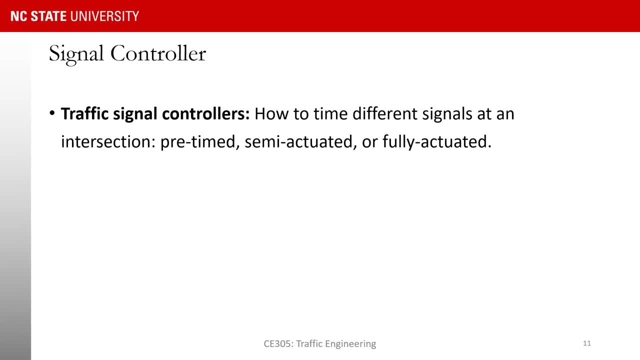 some of the streets are equipped with vehicle detectors and when they detect a vehicle, they're gonna provide green time for that movement and when the vehicle is gone, the green time is gonna expire. we also have fully actuated control when you have detectors on all movements and then the 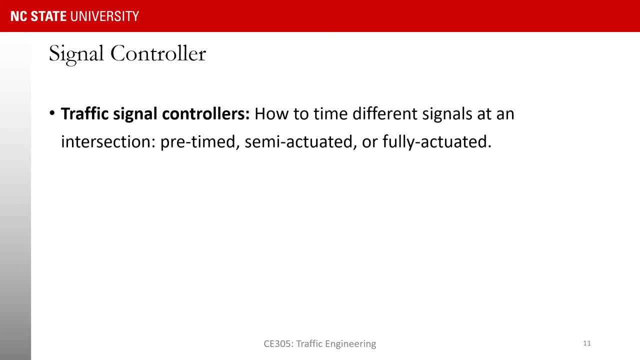 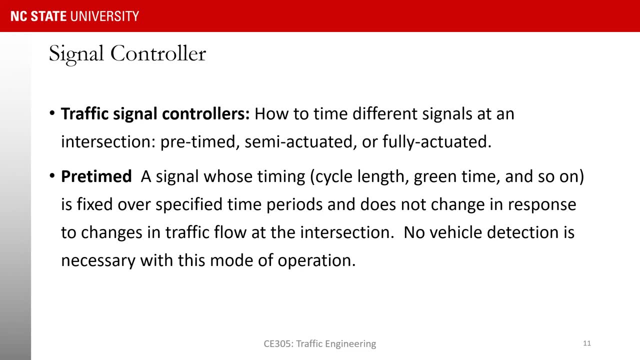 controller is going to provide green times based on detected vehicle time. it's set in different categories, like the first, ration and second and third and fourth and fifth, and so it's fixed during a specific period of time. and what this does- is it pictures you- that has been programmed, forried and comes out with a simulated signal. 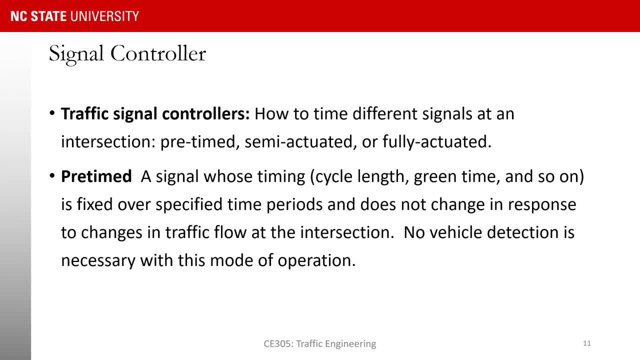 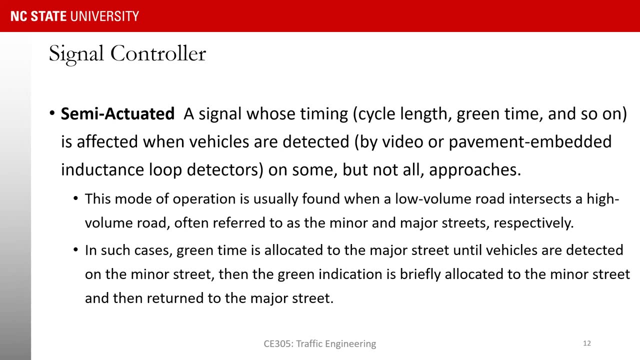 when you process the signal out, the three water regions get pushed up by the second channel. and, lastly, the four current are once again know that they are based on the thermal system-of-se- 같아 dense one semi-actuated. so you have detectors on some approaches and those detectors are 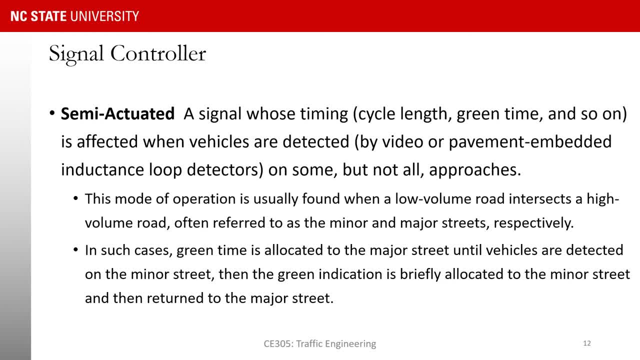 going to detect vehicle and, based on the detection, they're gonna provide signal to different movement. so if you think about a semi-actuated, I want you to think about some of the conditions that the semi-actuated control could be very useful, and that is when you have a major street intersecting a minor street. so 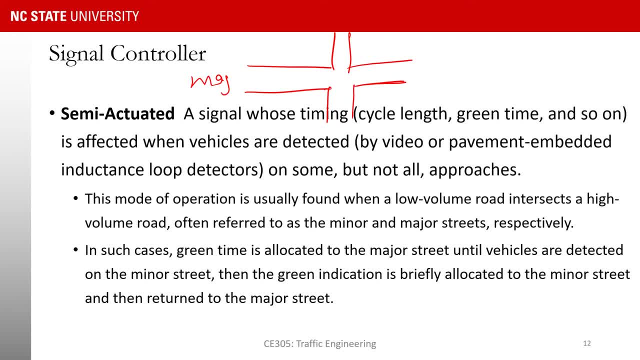 here I'm showing you this major street and then here I have the minor street. so if you have a major street, what you can do is that you can put detectors on the minor street, and what happens here is that we are going to provide the green time always. 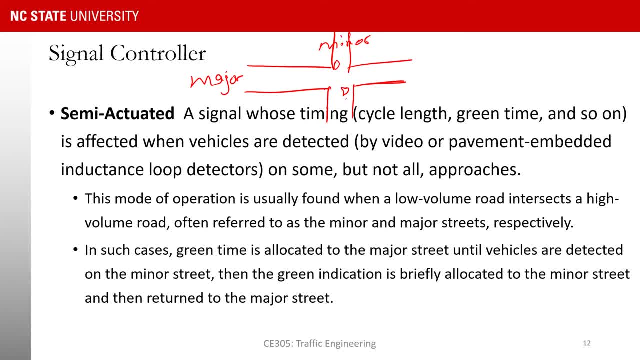 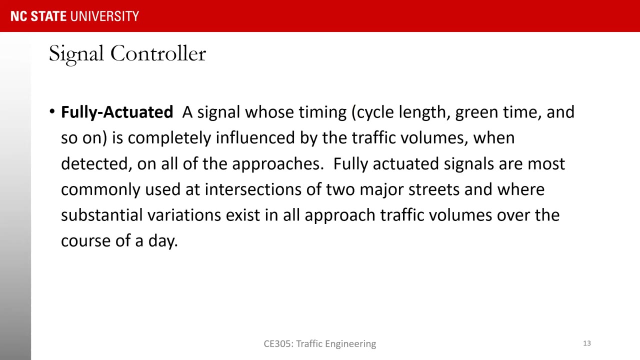 to the major street unless there is a detection in one of these detectors. if there is detection, the signal is gonna switch and we are gonna provide green to the minor street and when there is no more vehicles detected, the signal is gonna go back or the green is going to go back to the major street fully. 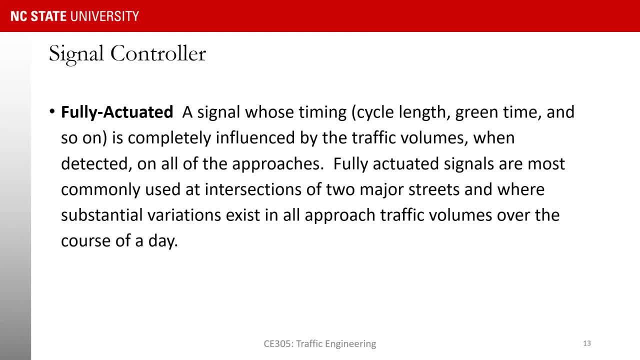 actuated. so in fully actuated, as I mentioned before, we are going to have vehicle detectors on all different movements. so what is going to happen there is that vehicle detectors are going to detect the presence of the vehicle and, based on the volume, they're going to allocate green to different movements. so usually what happens here? 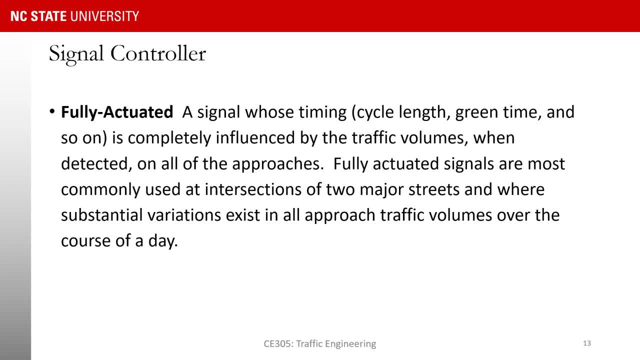 is that traffic engineer determines a minimum green to each approach. so when there is detection, that minimum green is going to be provided. so if one vehicle is there, or five vehicles, that minimum green is going to be given. now, if the detector keeps detecting more vehicles, that green duration is going to be given. so if the detector keeps detecting more vehicles, 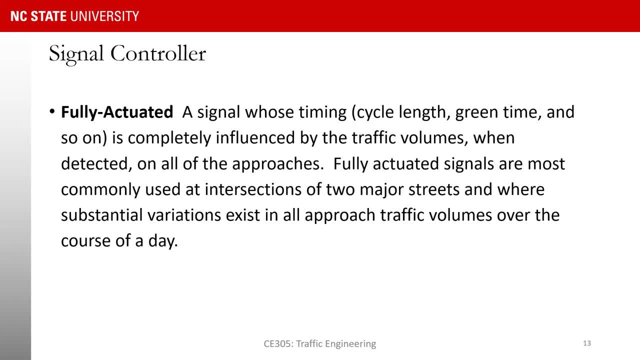 the green duration is going to be extended. more vehicles detected over time. the green is going to be extended over and over, let's say, two seconds. extension is going to be provided if you see more vehicles passing over the detector. so two things is going to happen: either there is enough vehicle, 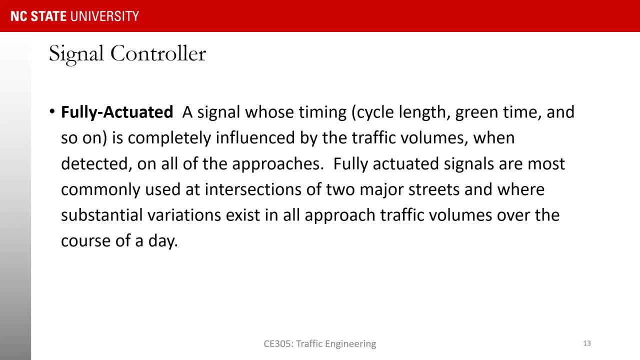 that the green time is gonna keep extending until it reaches a pre-specified maximum green time. at that time, the green time is going to be extended until it reaches a pre-specified maximum green time. at that time the green is going to be terminated or the detector does not detect a vehicle for some time. 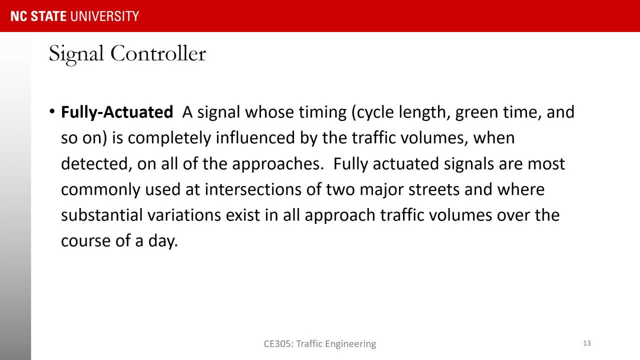 for a predefined duration of time. so there is a gap between vehicle arrivals and at that time the signal is going to be terminated. so if the signal gets to its maximum or the green time gets to its maximum and is terminated, we say the signal is maxed out. 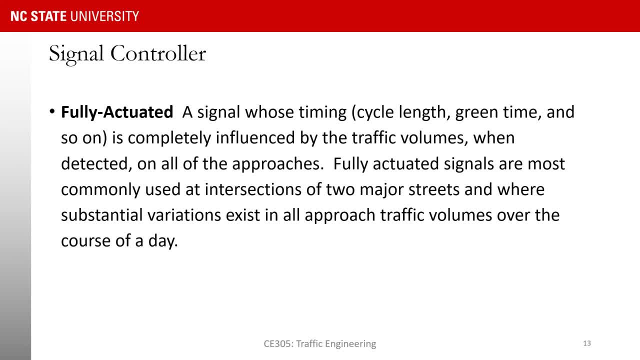 if the signal does not get to its maximum and is terminated because there was a large gap between vehicle arrival, we say the green phase is gapped out. so think about it: either the green, the green phase is going to be maxed out or gapped out, so when a green phase in a fully actuated system will be 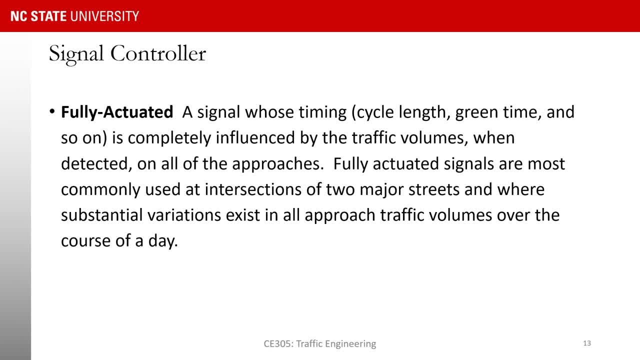 maxed out. when you have a lot of demand there and the maximum green is not enough to process all the demand, when is it going to be gapped out? when the demand is not high enough and some time after the minimum green, there is enough gap in the traffic. 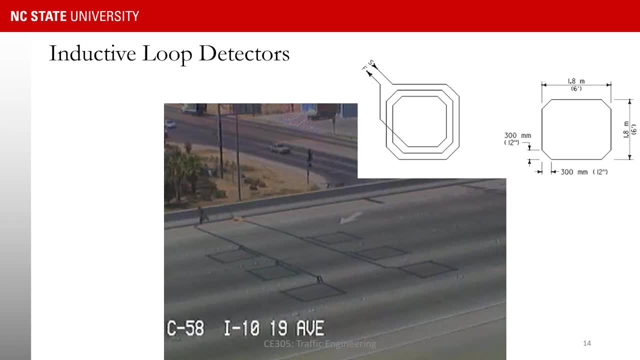 on this slide. um, we are seeing six loop detectors that are installed on a freeway facility. uh, it's this, it's pretty much the same thing on on intersections too. here you see six rectangles, or pretty much six feet by six feet squares. so we make tiny cuts on the pavement, we lay down the wire and then we cover it with epoxy or something like that, and 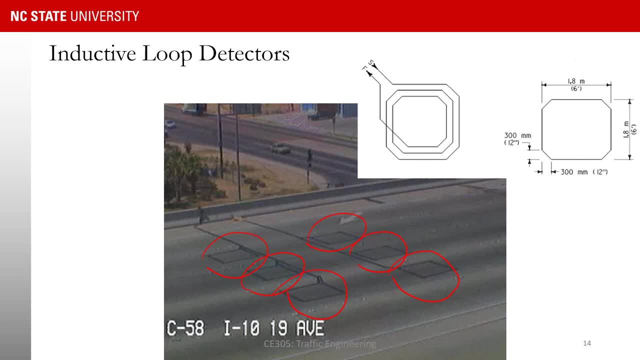 then the electricity is gonna go through the, the wires and, as a result, is gonna create a magnetic field. uh, and when vehicles go through that field, because they uh are are having a lot of metal, they're gonna create disruption in the field and the detector can detect that disruption and that's. 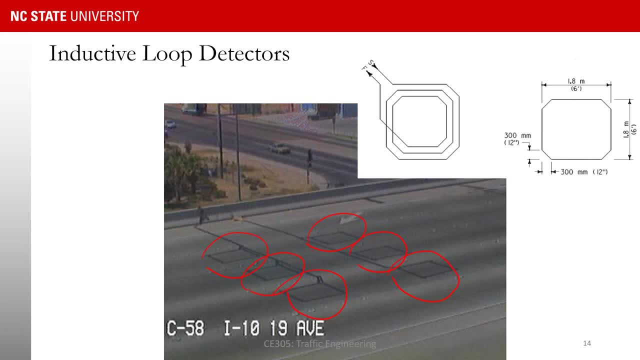 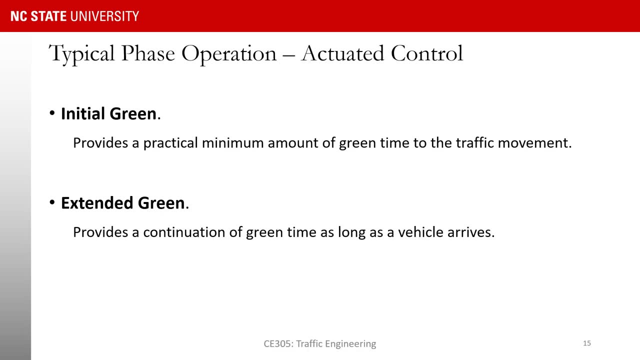 how a vehicle is is detected on on any any of these loop detectors. so again on this slide we talk about typical phase operations in actuated control. we have an initial green or a minimum green and then, based on vehicle detection, that green is extended either to the maximum green. 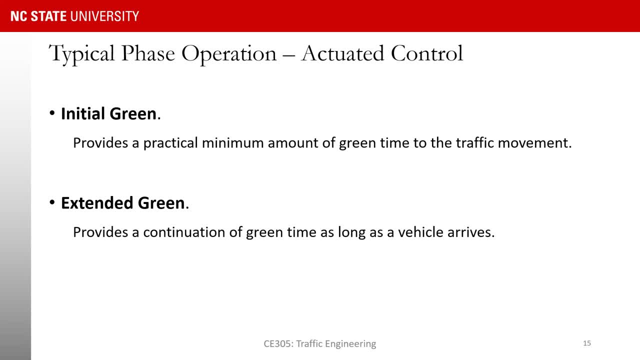 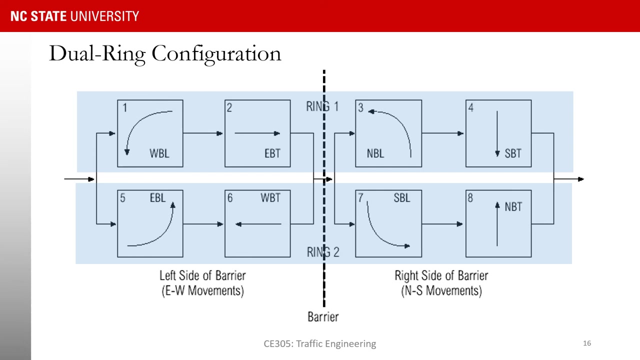 green when it is going to be maxed out or if there is not enough traffic demand that is detected by the detectors, we are going to have a gap out situation and the green extension is going to be stopped before hitting the maximum green. on this slide we are looking. 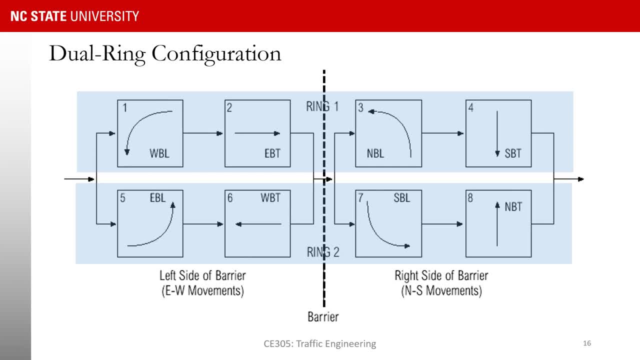 at a dual ring configuration and this is pretty much the way that traffic engineers show the phasing sequence or the possible or the possible phase sequences at a signalized intersections. here we have a intersection of two two-way streets and we are showing the dual ring configuration. 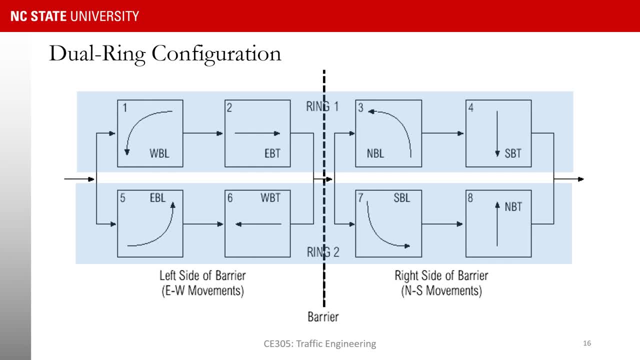 here. but before going through that, first we need to talk about how we have named these different movements. so you see WBL, EBL and things like that. so if you look at one intersection that I'm going to draw here, the way that we name the movements is based on the direction that they are headed to. so if you 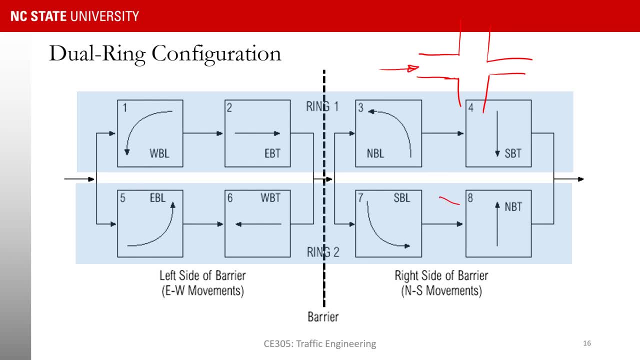 have vehicles that are going from west to east. we call that east bound, so this is east bound movement and we pretty much call this entire approach east bound approach. so we are going to have south bound approach, we are going to have northbound approach and we are going to have westbound approach, and then when? we think about different movements that we can have, or different territory as well. we have many kind of. should we look at the truth of that intersection, such as J and the other~ else? Why has not that intersection of here A and A is the best point of the intersection. 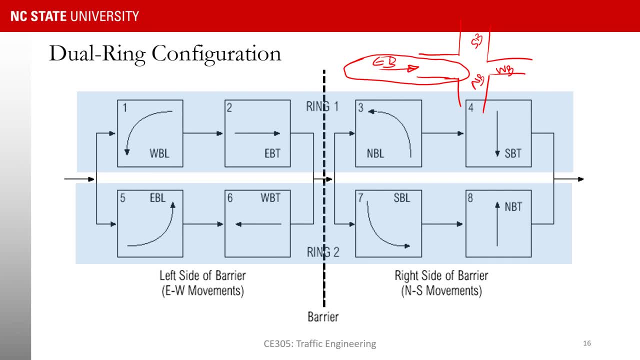 so sometimes those are no pure solutions and that is whyibo this is a different demonstration and we can dezёлette any specific single placement of any Delta in terms of location, towards different locations or however you think about things like that, turning movements. we are going to continue or build on what we have seen so far, so I'm going. 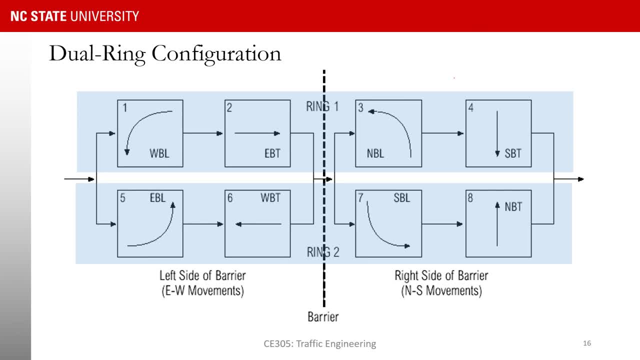 to get rid of this and let me just focus on eastbound approach. so if you have vehicles that are going through, we call them eastbound through. if you have vehicles on eastbound approach that are making a left turn, we call them eastbound left, and if you have vehicles that are making 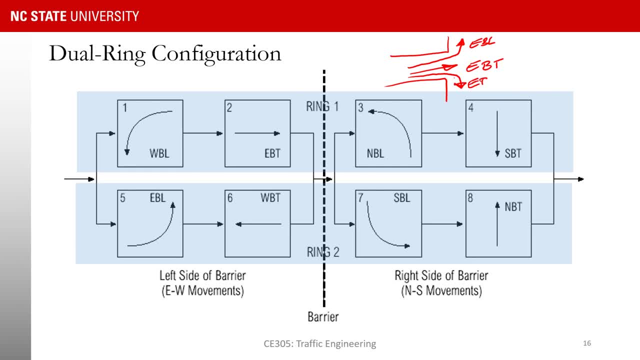 a right turn. we call them eastbound right. so what if we have a lane that has both eastbound through and eastbound right? we call it eastbound through right. and pretty much the same convention is used to call other movements at a signalized intersection. so here you are, seeing those different movements I have: westbound left, eastbound left. here I have 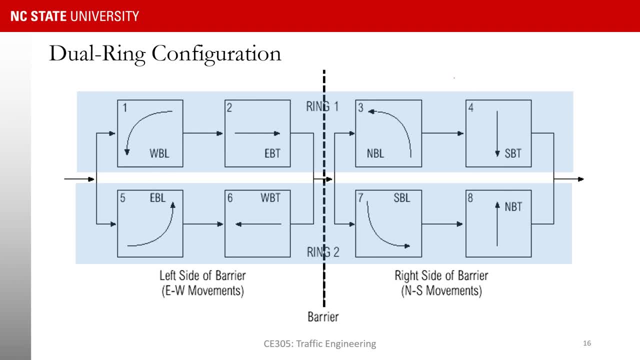 eastbound through, westbound, through, northbound left, southbound left and southbound through and northbound through. so I have two rings here, one on the top and one on one on the bottom. I also have something here that I call it a barrier. so a barrier is telling us that no movement on one side of the barrier can go with any movement. 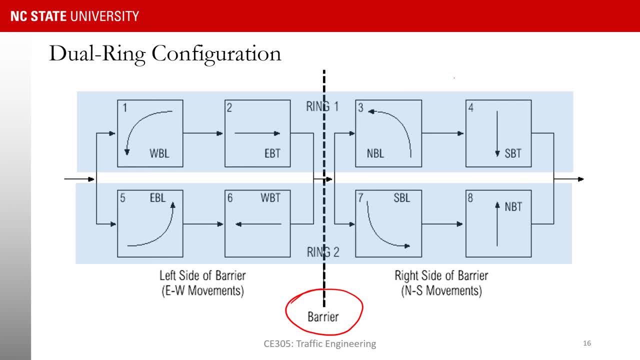 on the other side of the barrier. for, for example, if you select movement number two and you select movement number, movement number eight, so eastbound through and northbound through, these two movements cannot go at the same time because they are conflicting. so any movement on one side of the barrier. 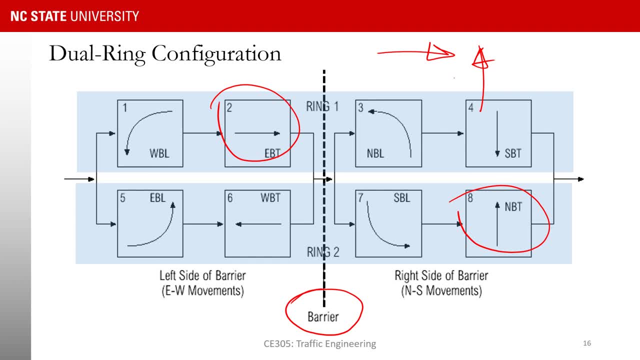 cannot go with any movement on the other side of the barrier, so we have two rings. this is ring number one and this one is ring number two. any movement on ring number one can go with any movement on ring number two at the same time, as long as they are from the same side.